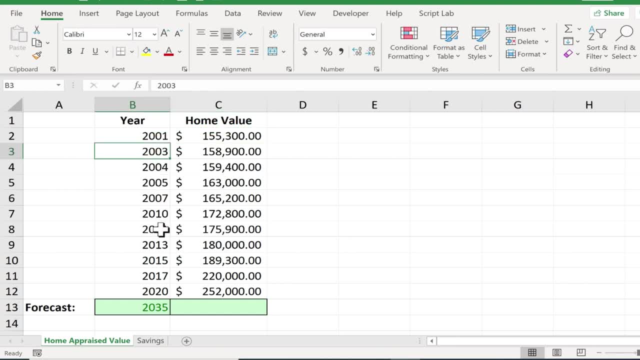 at the time And then maybe every year or two or three, the house got appraised. But each of these years has a different home value for the home. And these years are all in the past, of course. But what about the future? Is there a way to kind of forecast what the 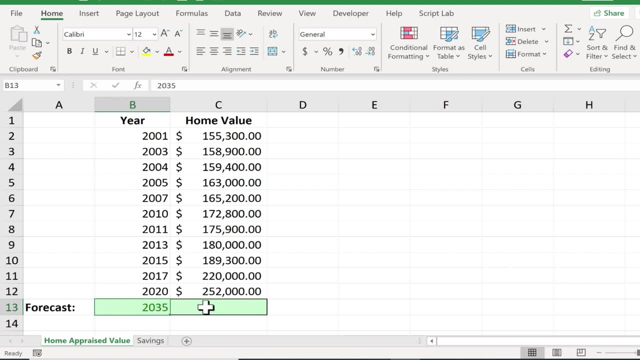 value of this home will be in 2035?. Now, before I show you how to do this in Excel, just know that this is limited. Obviously, Excel doesn't know that much about home values. It doesn't know how real estate appreciates. 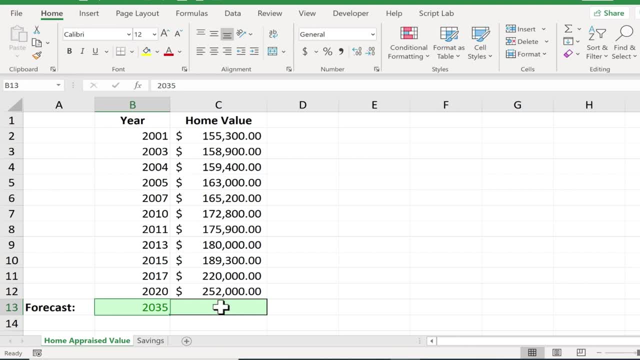 and it doesn't know the neighborhood that I live in or things like that. There's all sorts of variables, But using the information that we do know, Excel can make an educated guess about the future. So here in this blank cell, I'm just going to click and then type. 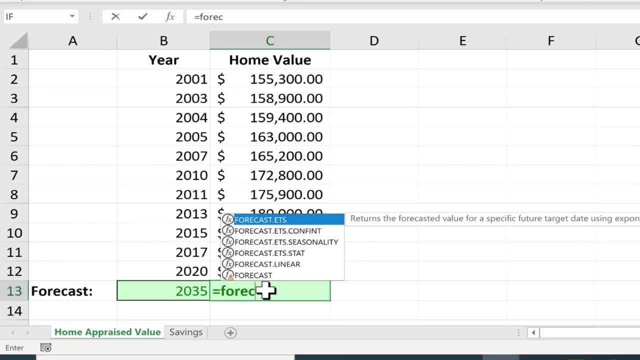 the equals sign and I'll type in the function forecast. Now you'll notice there are six different forecast functions. They're all pretty similar, But if you know that what you're looking at is a linear model, you could choose Forecast. 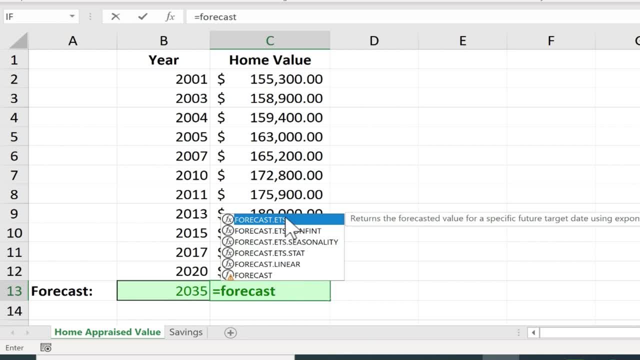 Linear. If you know that what you're looking at is an exponential model, you could use Forecastets, And there's all of these other slightly different versions of the forecast function. If you're not sure which one to use, just stick with Basic Forecast, So that's. 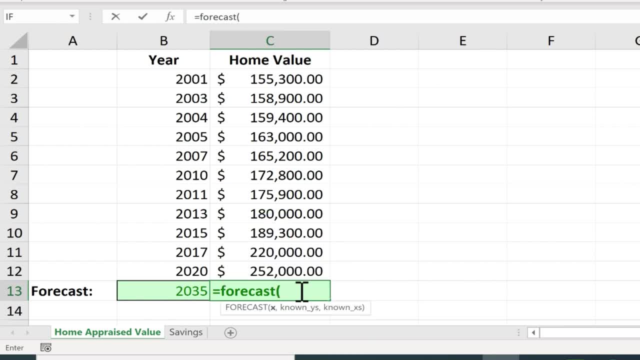 what I'm going to do. After typing in Forecast, I'll just put a left parentheses And you can see what Excel is looking for. It's looking for an example of some sort of a forecast: an X number and then comma, and a known Y comma and then a known X. So this can be really. 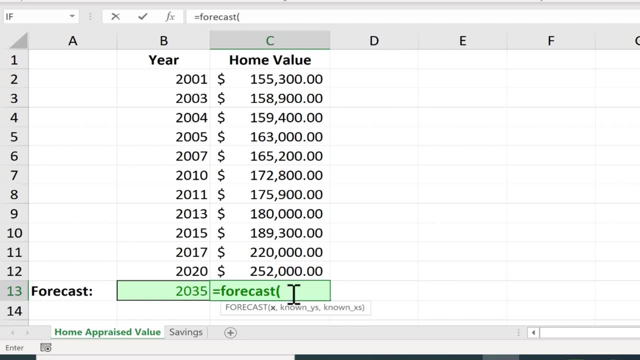 confusing at first, But basically the forecast, I want it to be based on the year 2035.. So I'm going to click on 2035.. That will become the X, So I click on 2035.. Now I didn't really click on. 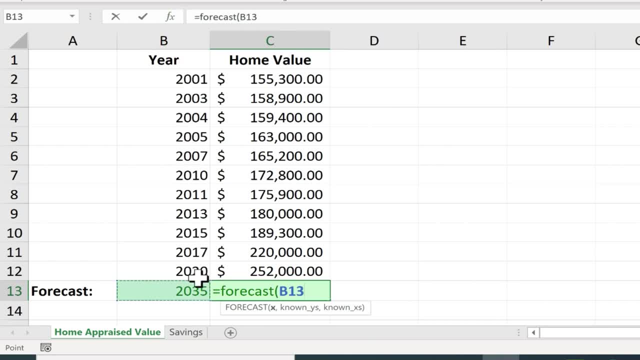 the number. I actually clicked on the cell, cell B13.. So anything that I type in B13, that will become the X. Now I type comma and the known Y. Okay so, since this is X, the Y must be this. 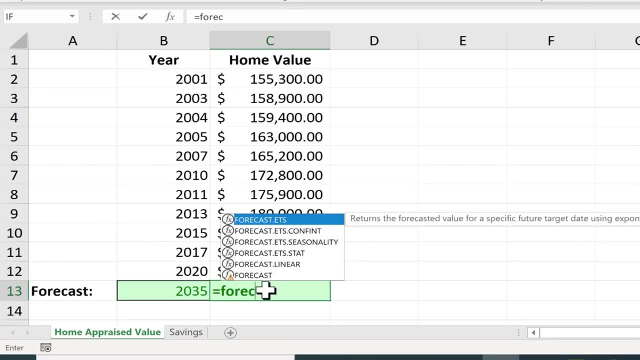 the equals sign and I'll type in the function forecast. Now you'll notice there are six different forecast functions. They're all pretty similar, But if you know that what you're looking at is a linear model, you could choose forecast. 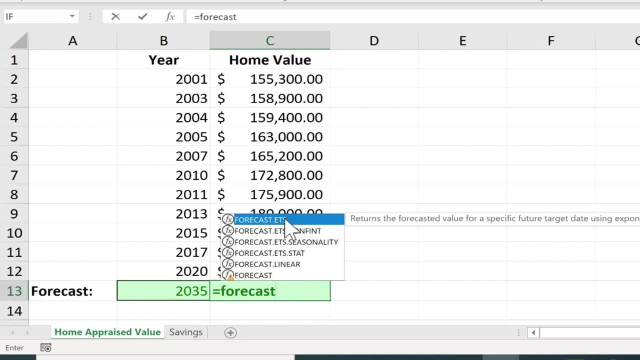 linear. If you know that what you're looking at is an exponential model, you could use forecastets. And there's all of these other slightly different versions of the forecast function. If you're not sure which one to use, just stick with basic forecast, So that's. 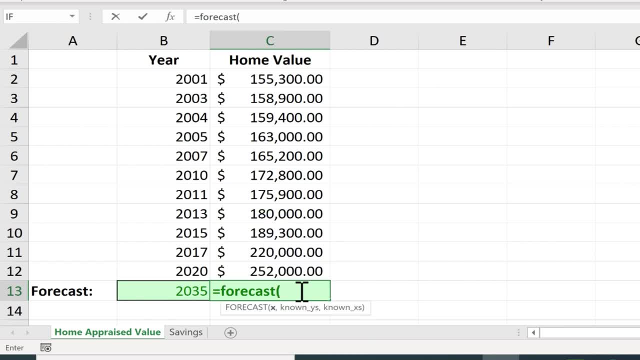 what I'm going to do After typing in forecast. I'll just put a left parenthesis and you can see what Excel is looking for. It's looking for an exponential model. So I'm going to click on the x number and then comma, and a known y comma and then a known x. So this: 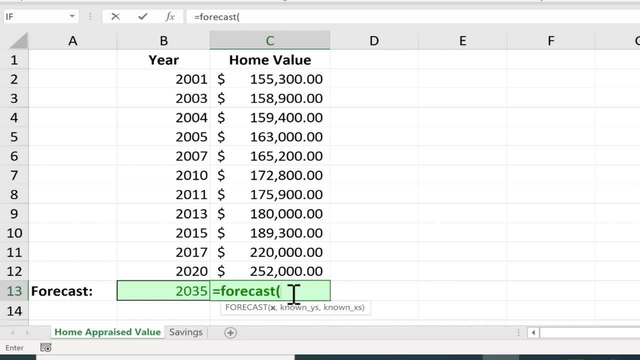 can be really confusing at first. But basically the forecast. I want it to be based on the year 2035.. So I'm going to click on 2035.. That will become the x, So I click on 2035.. 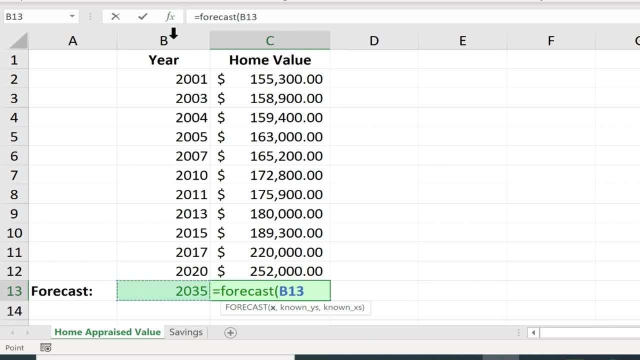 Now I didn't really click on the number. I actually clicked on the cell, cell B13.. So anything that I type in B13, that will become the x. Now I type comma and the known y. Okay, so since this is x, the y must be this information. 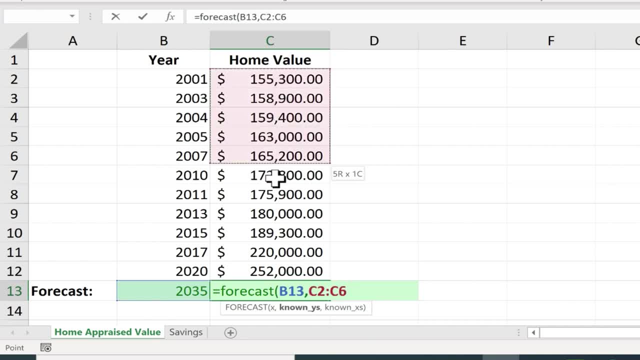 here And it is So. this is the information that we know. We know what the past appraisal values have been, So I just clicked and dragged to select all of the past appraisal amounts And now I'll put a comma in. And now it wants the known x's. So this is x. What are the? 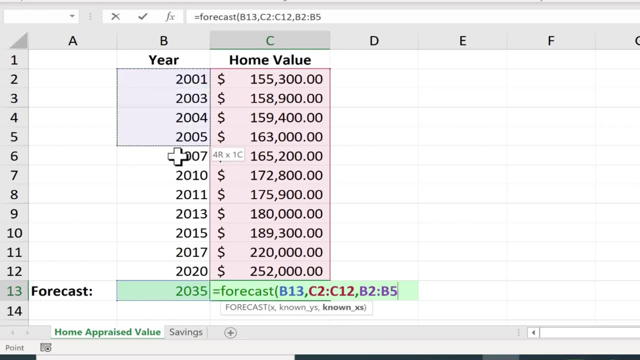 known x's Well all of these years. So I click and drag to highlight all of the past years And then I should put in a right parenthesis and tap enter on the keyboard And it calculates what Excel thinks my home will be worth in 2035, based on past results. Okay, let's try that again This time I'm 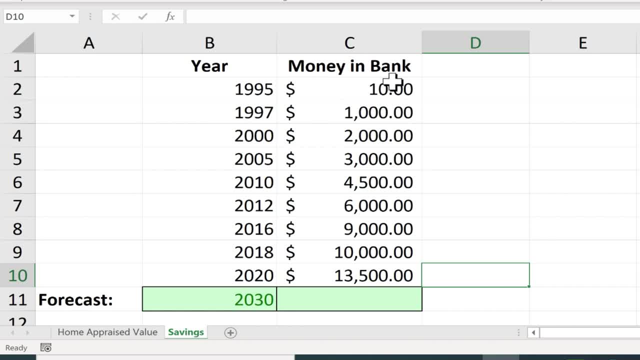 going to go to the savings spreadsheet And this again is limited And there's going to be some flaws in this. Excel doesn't know my saving habits and things like that, But in 1995, I had $10 in the bank. In 2005, I had $3,000.. I would follow the same pattern. 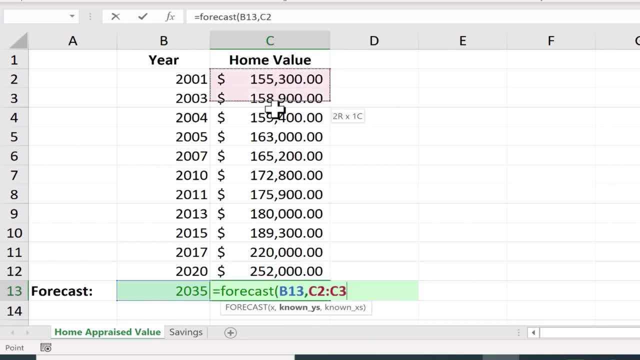 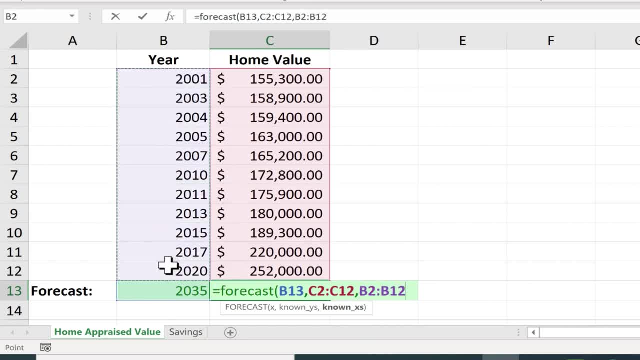 So I click and drag to highlight all of the past years, And then I should put in a right parenthesis and tap enter on the keyboard And it calculates what Excel thinks my home will be worth in 2035, based on past results. Okay, let's try that again. This time I'm going to go to the 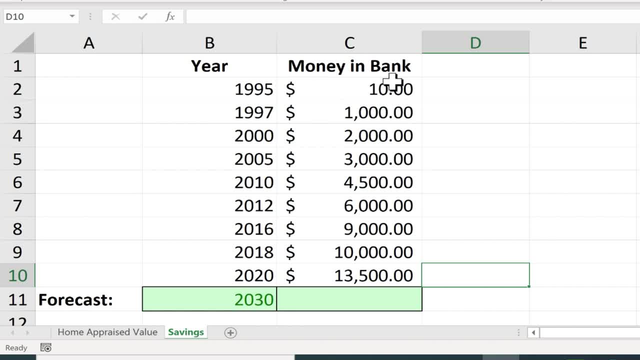 savings spreadsheet, And this again is limited And there's going to be some flaws in this. Excel doesn't know my saving habits and things like that, But let's say in 1995 I had $10 in the bank. In 2005 I had $3,000.. I would follow the same pattern. 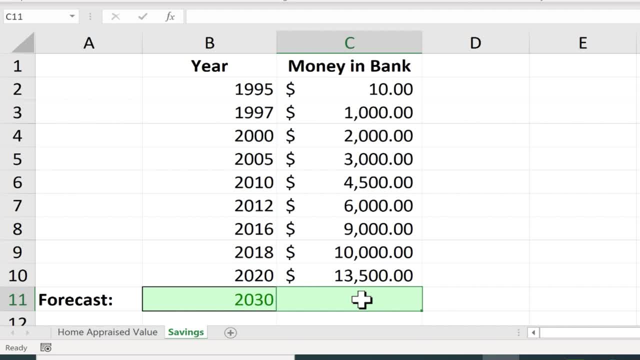 as before, I would go here to this cell and click and type equals forecast, left parenthesis. What's the X? What is this forecast based on? Well, it's based on the year 2030.. So I click on that cell, B11.. Type the comma. What's the known Y of this data? If this is X, then this is Y. 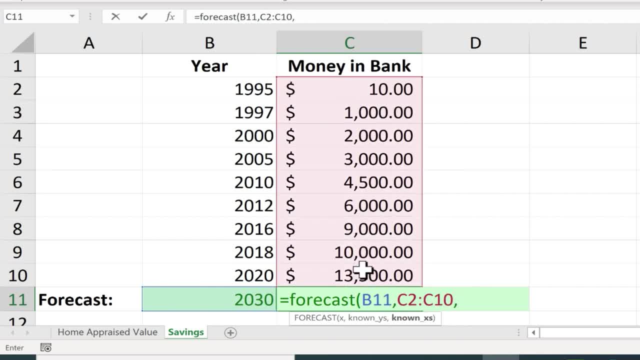 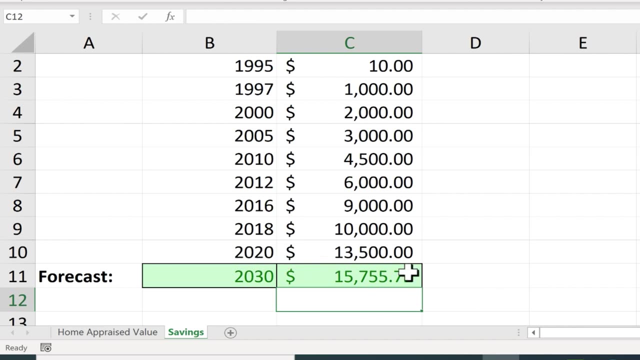 So I'll click here to select all of the Y comma and now the known X. Well, here are the known X's, So I click and drag to select those Put in the right parenthesis, Tap enter. And apparently that's what I would have in 2030.. That's not a lot of savings for 10 years And, like I said, 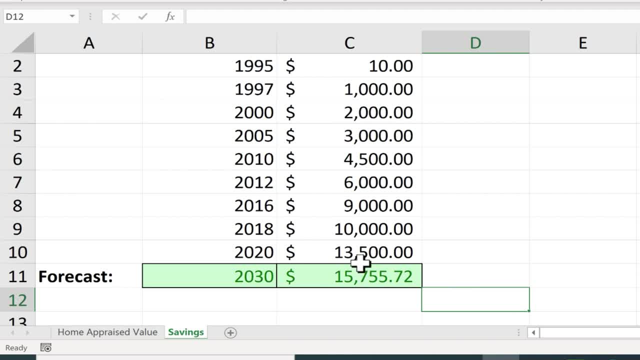 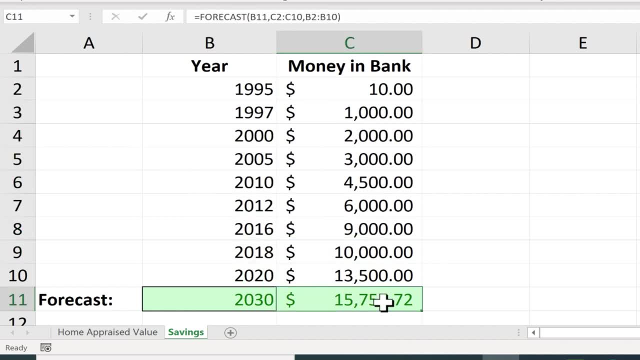 this forecast ability is pretty limited, But Excel is doing its best to figure out. okay, given these numbers and their relationship to these numbers, this is what Excel is going to be able to do. So I'm going to click here to select all of the Y. 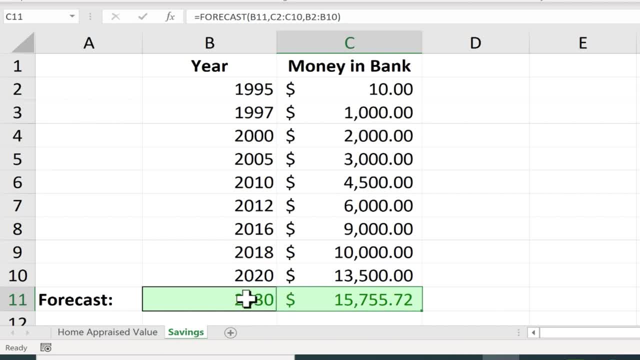 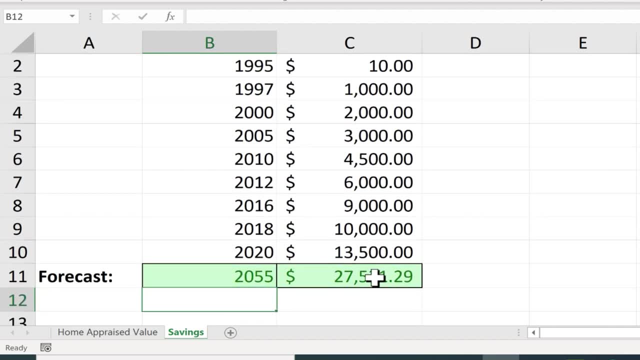 comma. and now this is what Excel expects for 2030.. Now notice that you can go in here and change from 2030.. I could put 2055.. Tap enter And the model updates, the forecast updates and this is. 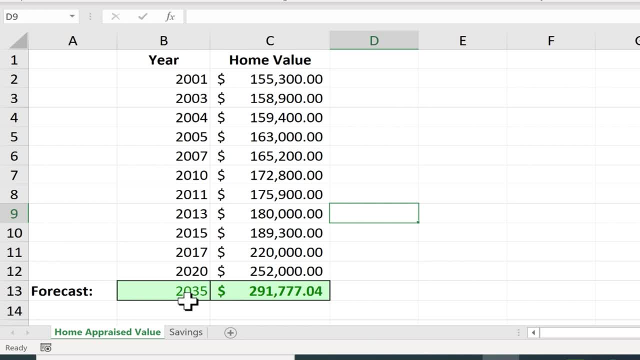 now the expected amount. I can do the same thing with home appraised value, So I could change this from 2035.. What about 2055?? I'll tap enter And I can see: oh, that is now the expected amount.